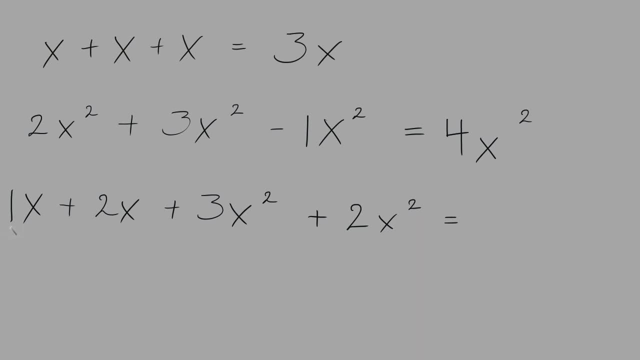 coefficients for the terms that are alike. 1 plus 2 is 3.. We'll put down our 3 and keep the same variable of x. These two terms get added on to the next two terms of 3x squared plus 2x squared. So because they are like terms, we can add the coefficient 3 plus 2.. 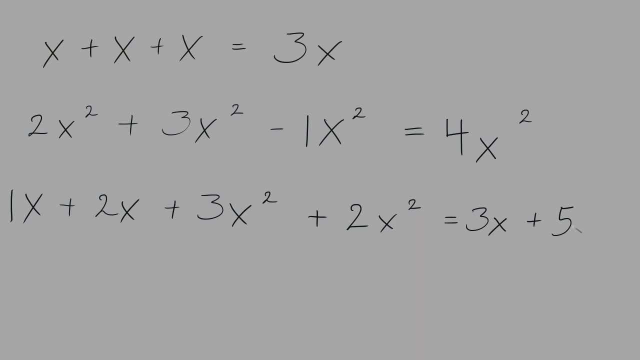 3 plus 2 is 5.. We will keep the same variable and the same exponent. So the answer is 3x plus 5x squared 4x to the power of 4 subtract 3x to the power of 3 plus 2x squared subtract 1.. In this example, the 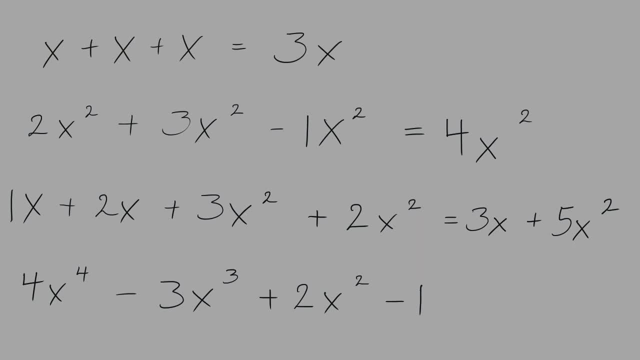 we have three terms with the variable x, but because of the different exponents in each term they are not like terms and no variable or exponent at all on the minus one. so these terms cannot be combined. so we can't do anything, we just leave it the way it is. 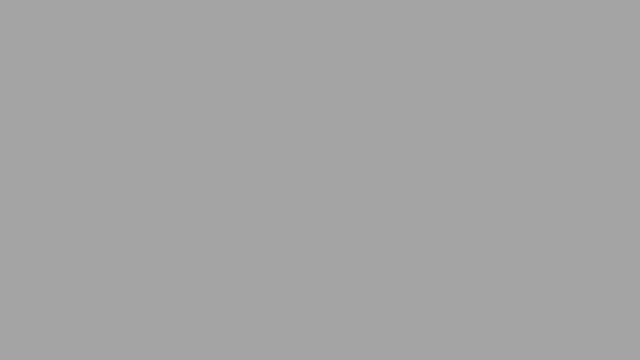 so we have learned that when adding or subtracting variables with exponents, you must have exactly the same variables and exactly the same exponents in the terms that are being added or subtracted. this is called combining like terms. next we'll be multiplying variables with exponents. 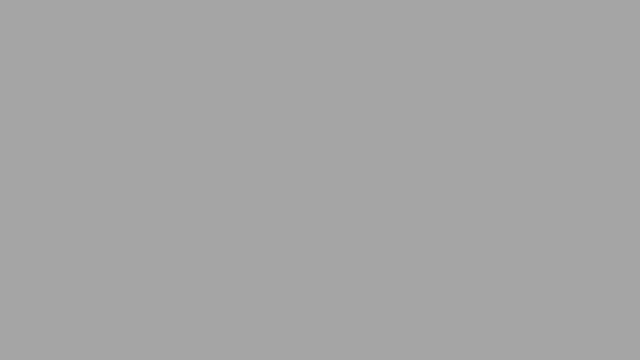 when the terms being combined are multiplied, the variables must be the same but the exponents can be different. so let's say you had something like x to the power of three and it's multiplied by x to the power of 4.. This is the same as saying x, 3 plus 4.. You just add the exponents, So the answer is x to the power. 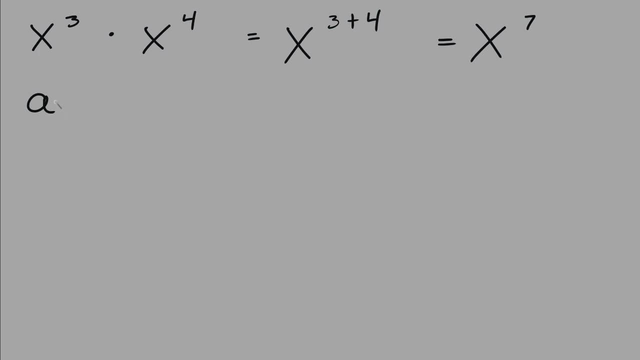 of 7.. Now let's say you had something like a to the power of 3 and it's multiplied by a to the power of 5.. This is the same as saying a 3 plus 5, which is going to equal a to the power of 8.. 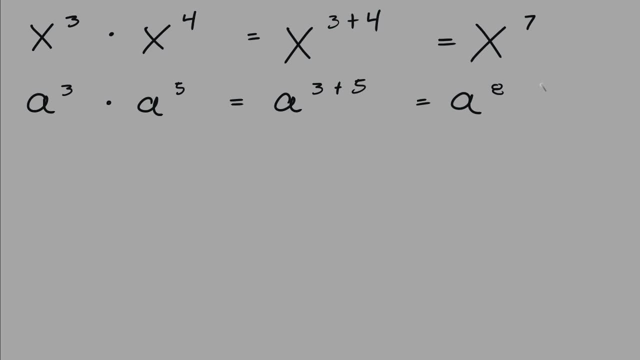 And let's say if you had a coefficient in front of the variable like 2x squared and it's multiplied by 2x to the power of 3. In this case you would multiply the coefficients. So 2 times 2 is 4.. Put down your variable x and then you add your exponents. 2 plus 3 is 5.. 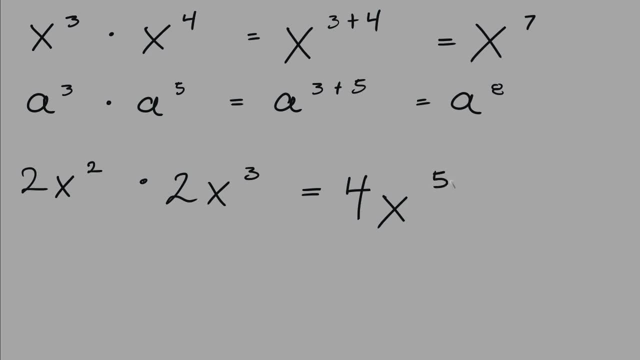 So the answer is 4x to the power of 5.. Let's say we had 3a to the power of 3 multiplied by 4a to the power of 4. And you multiply your coefficients 3 times. 4 is 12.. Put down your. 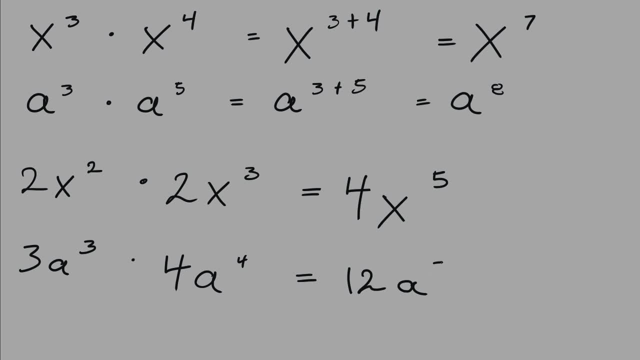 variable a, 3 plus 4 is 7.. So the answer is x to the power of 5. And the answer is 12a to the power of 7.. 2a squared, a to the power of 3.. And then 3b squared, And then b to the power of 3.. 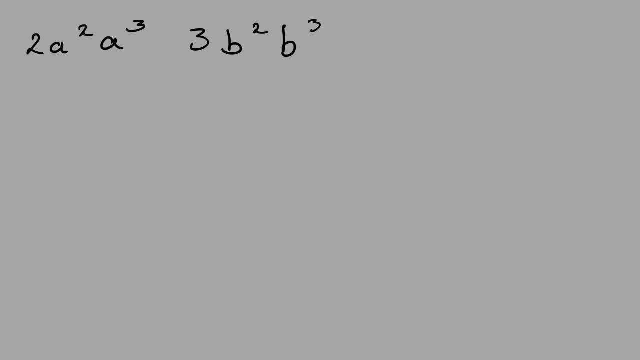 Because they're all multiplied together. it doesn't matter which order you do it in, So you can rewrite the question 2 times 3.. Times a squared Times a to the power of 3.. Times b squared Times b to the power of 3.. 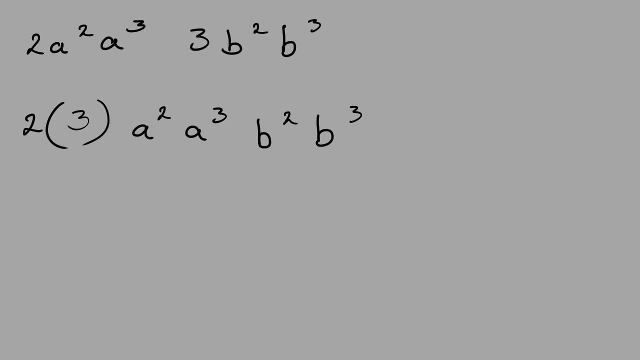 So the next thing you can do is you can multiply the 2 times 3, which is 6.. And then, because you have the same variable 2 times, what you do is you add the exponents, So it's a, to the power of 2 plus 3.. 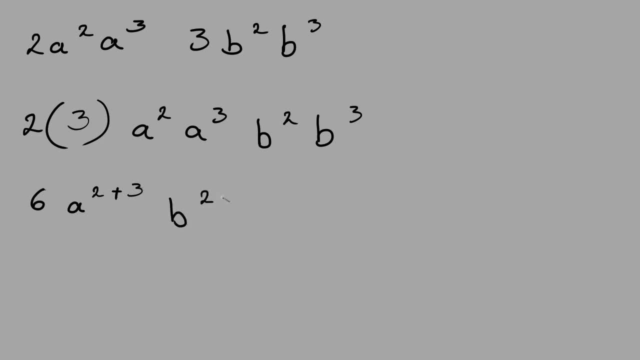 And then b to the power of 2.. 2 plus 3.. So then you can add the exponents together. You will have 6a to the power of 5. And then b to the power of 5.. So this is fully simplified. 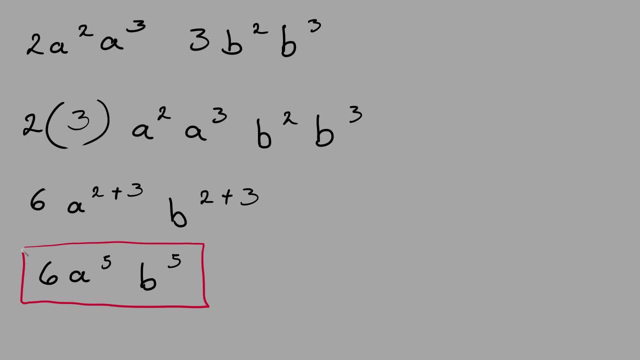 You cannot multiply the a and b together because they are not like terms. So let's try another one. Let's say you have 2a squared b, squared c to the power of 3.. And then you have 4a to the power of 3, b to the power of 2, and c to the power of 4.. 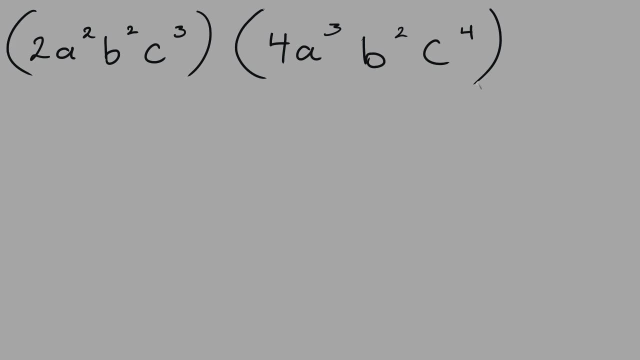 So we know we can rewrite the question to put the coefficients together. So we can say: 2 is multiplied by 4. Then we have the variable a, which is squared, And then we have another, a power of 3. So we can put those together and say a. 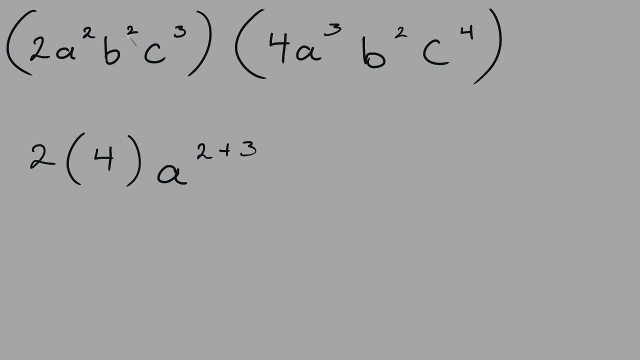 2 plus 3.. And then we have b to the power of 2, and another b to the power of 2.. So we can say b, 2 plus 2.. And then we have c to the power of 3.. 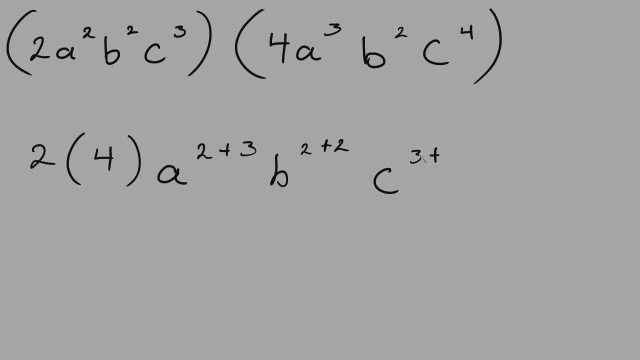 And over here we have c to the power of 4.. So we can say 3 plus 4.. So we'll go ahead and multiply 2 times 4, which is 8.. Then we have a: 2 plus 3 is 5.. 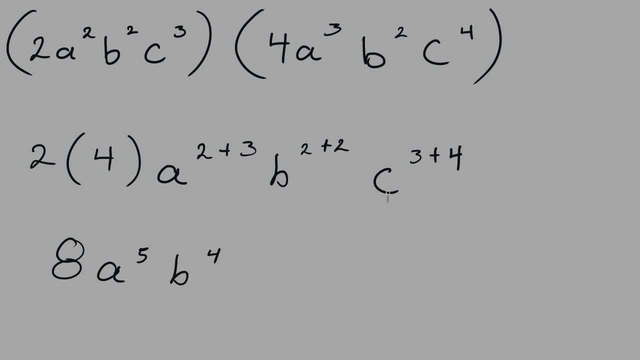 Then we have b 2 plus 2 is 5.. Then we have a 2 plus 3 is 5. is 4. and we have C 3 plus 4 is 7, and this is fully simplified. so to multiply: 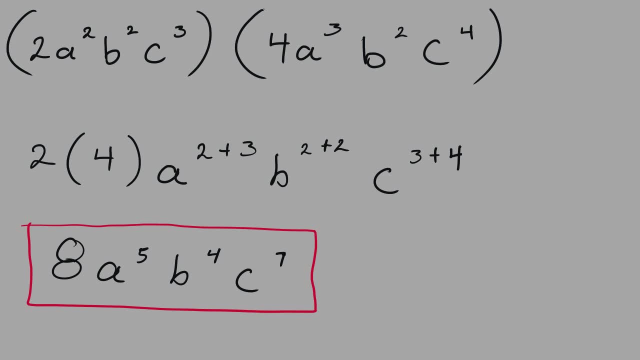 variables with powers. we simply multiply the coefficients and then add the exponents on the variables that are alike, and I wanted to explain the difference between negative 3x raised to the power of 2 and negative 3x in brackets raised to the power of 2. so this exponent of 2 only applies to the. 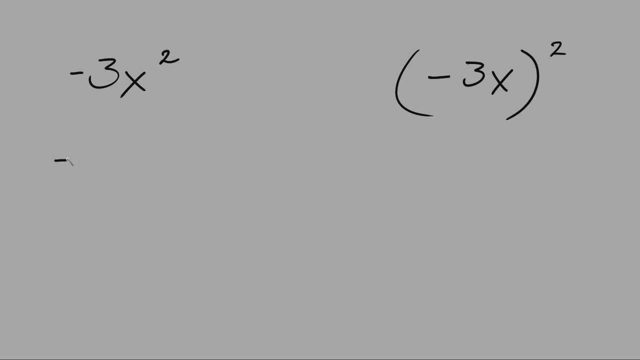 variable that is beside it. so it means negative 3 times X times X, and this power of 2 will apply to everything within the brackets. So it means negative 3x times negative, 3x, Negative 3 times negative, 3 is positive 9 and x times x is x squared. 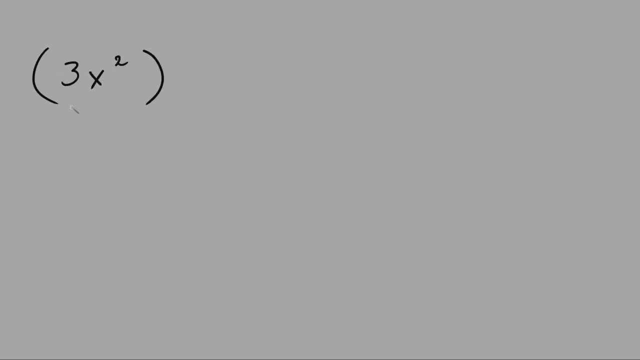 Three x squared in brackets, raised to the power of 4.. What you do is you distribute the 4 to the coefficient of 3 and to the power of 2.. So 3 to the power of 4, the variable is x, and when you have a power raised to a power, 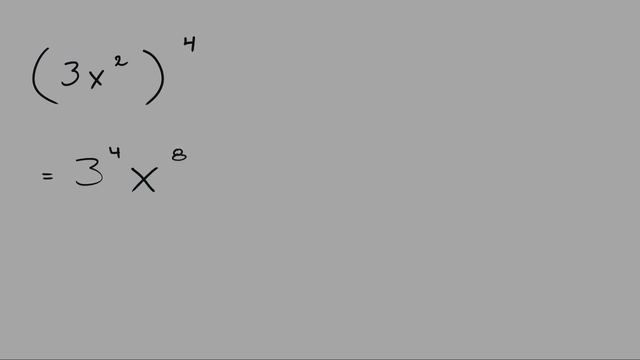 you multiply them, So 2 times 4 is 8.. So 3 to the power of 4 is 3 times 3, which is 9 times 3, which is 27 times 3, which is 81. So you will have 81.. 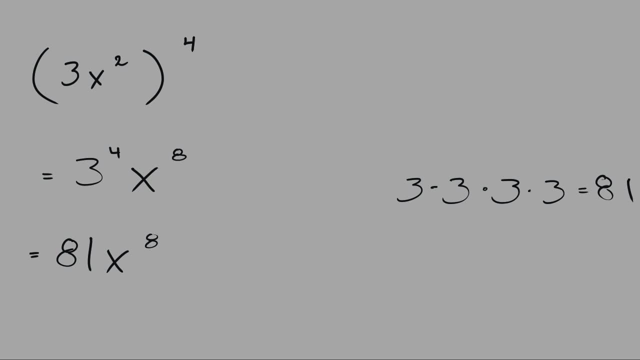 Your variable is x to the power of 8.. Okay, To learn more about exponents, you can watch my video called the laws of exponents. So let's talk about dividing variables with exponents. So this is like working with fractions. Let's say you have x to the power of 6 on the top, divided by x to the power of 4.. 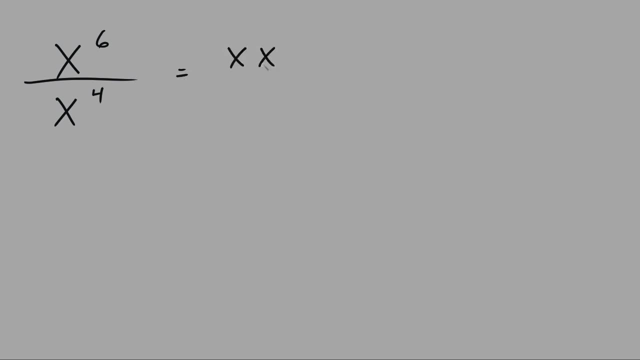 This is equal to saying x times itself, 6 times on the top and x times itself 4 times on the bottom. So when you have the same variable on the top and the bottom, you can cancel them out. So we cancel out 4 on the bottom, we'll cancel out 4 on the top. 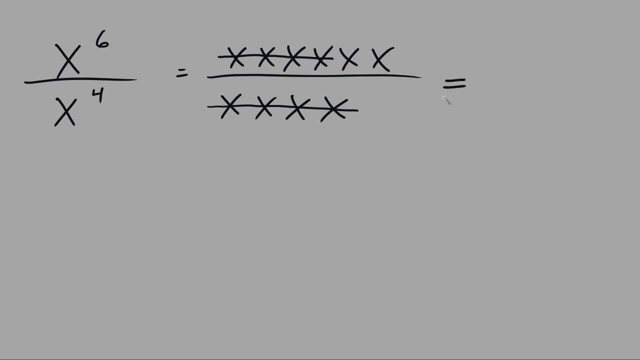 So we're left with x times x on the top, which is the same as saying x squared. Or you could simply subtract the exponents: 6, take away 4 is going to leave you with x to the power of 2.. 14 x to the power of 2 divided by 7, x to the power of 4.. 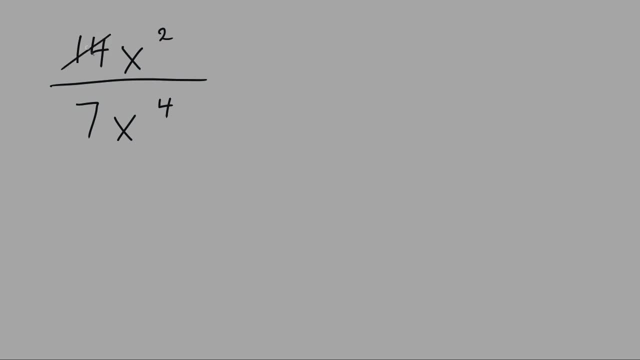 Now 14 is divisible by 7.. 14 divided by 7 is 2.. 7 divided by 7 is 1.. So we will have 2 x squared over 1 x to the power of 4. And we have the variable x on top and bottom. 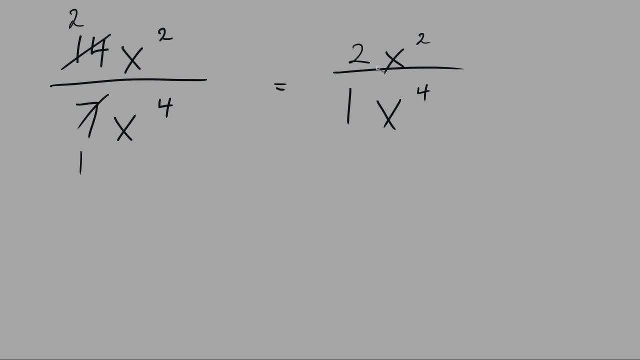 So we will subtract 2 from 4.. So the x to the power of 2 will get cancelled out and 4 subtract 2 will become 2.. So we're left with 2 on the top, and on the bottom we have 1 x or just x. 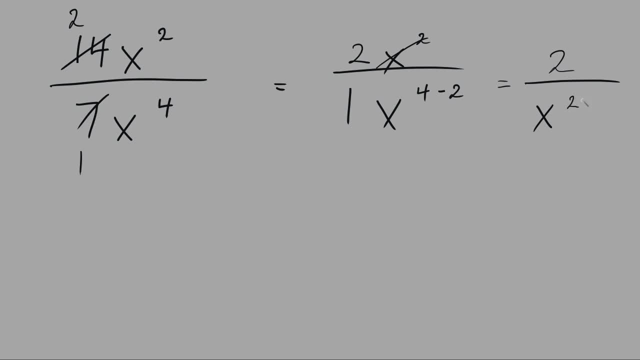 4. subtract 2 is 2.. So x to the power of 2. 8, x to the power of 12 divided by 64.. x to the power of 2.. x to the power of 3.. 8 and 64 are both divisible by 8..